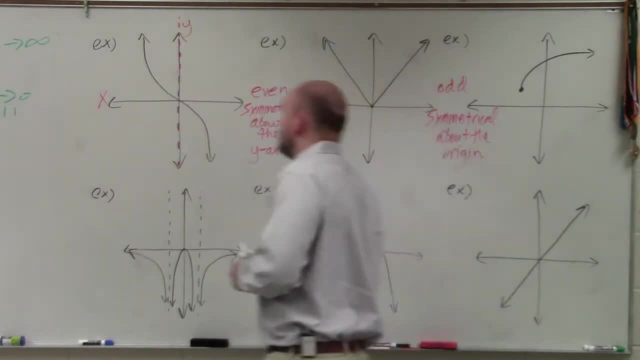 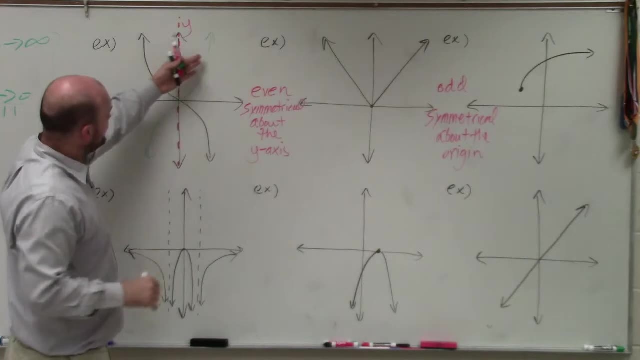 However, if I reflect the graph over the y-axis, I'm now going to produce something that's going to look like this: And if I now take this graph, the green graph, and reflect it over the x-axis, which would represent the origin, reflecting over the y, 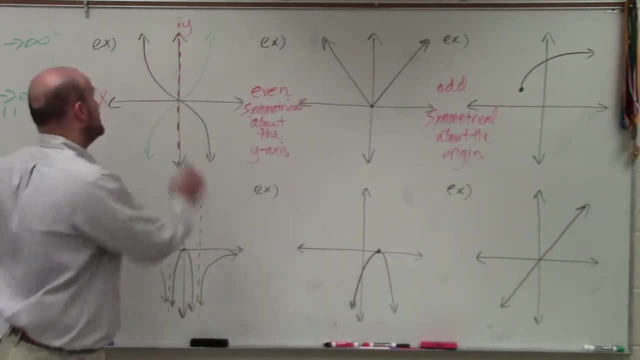 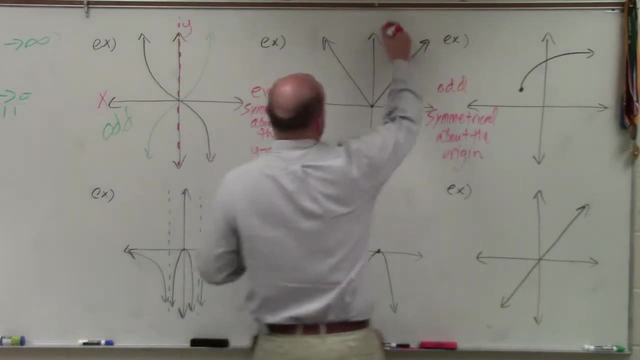 and the x-axis, I would produce the exact same equation. So therefore this graph is odd Over here. you can see that now, when I take my line of symmetry about the y-axis, that dotted line cuts this v graph, the absolute value. 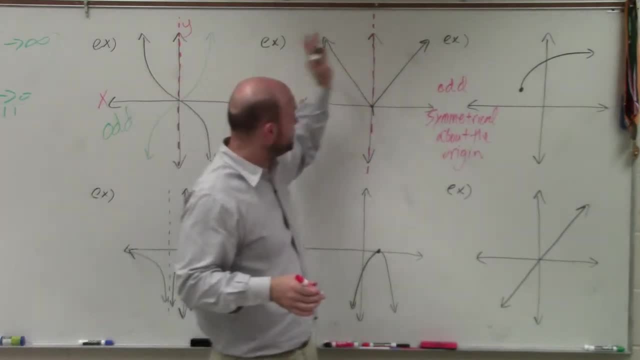 graph directly in half, What is the exact same as on the left side. if I reflect over, it's going to be exactly over the right-hand side. So therefore, this is an example of, even because it's symmetrical. It's symmetrical about the y-axis. 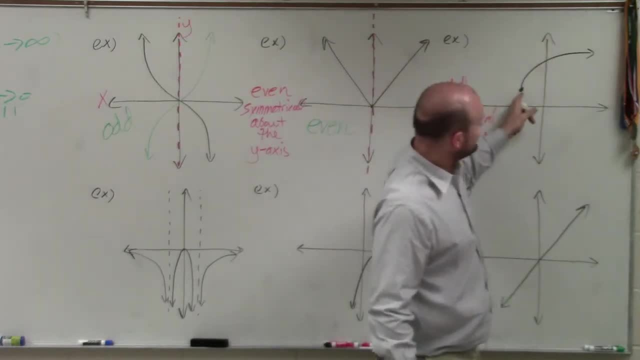 Over here. if I cut the graph, you can see the graph stops here and it goes infinitely there. So a line about the symmetry of the y-axis is not going to cut the graph in half. But what about if I reflect it over and then 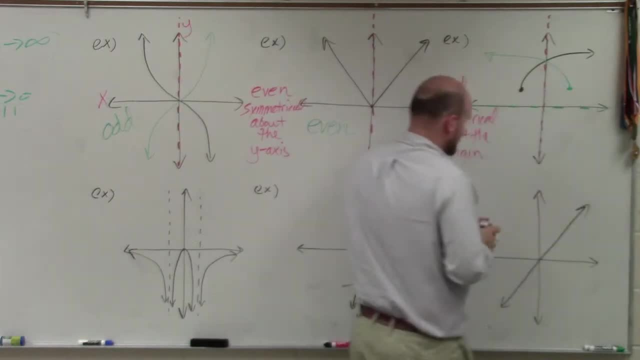 reflect it over the x-axis. Well, if I do all of that, then I'm going to have a graph that's going to look like this, which again does not take me back to my original graph. So, therefore, this is an example of neither. 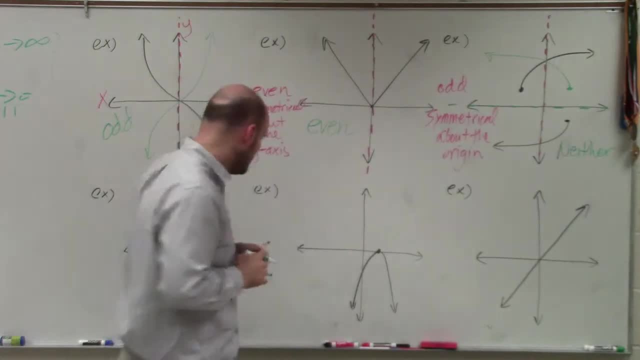 meaning it's not even nor odd function Over here. now this one looks kind of crazy. You have these asymptotes, You have all this crazy stuff going on. However, if you dissect what's going on to the left of the y-axis, as well as what's 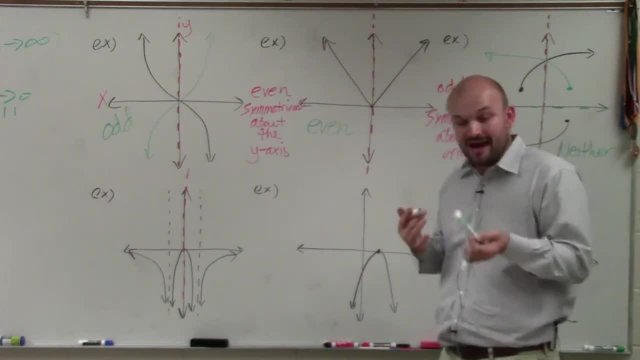 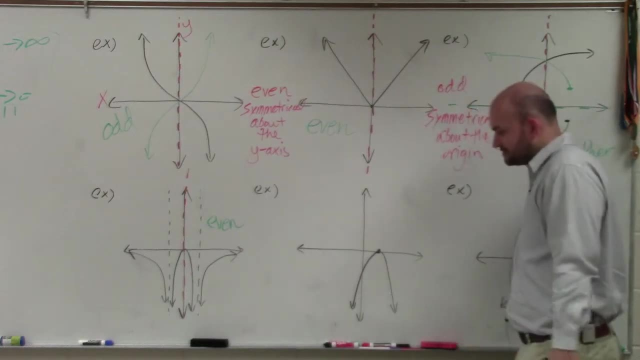 going on to the right of the y-axis, you can see that the graph is symmetrical about the y-axis. So since it's symmetrical about the y-axis, this graph is even Now. this one gets students confused quite a bit because 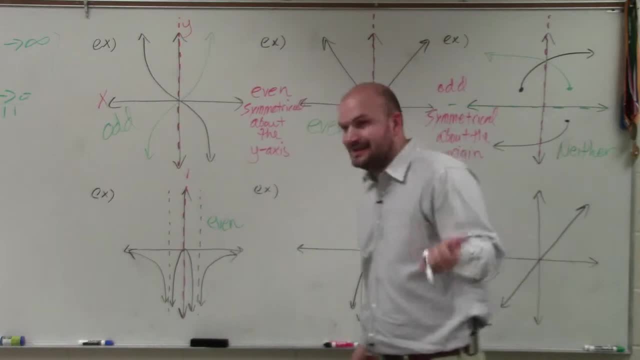 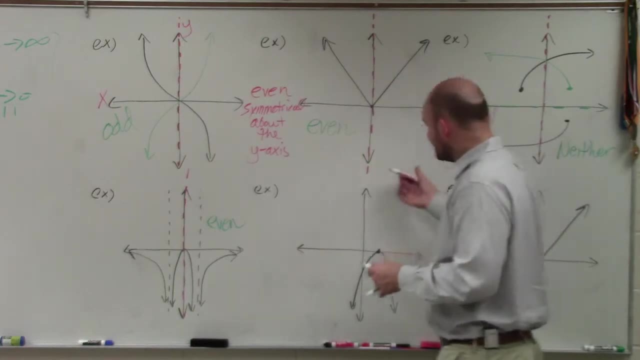 They see a parabola and they know, hey, parabola is an even function. But however, the way that this parabola is written, it's written, it's been shifted over to the right. So if I was going to use a line of symmetry, 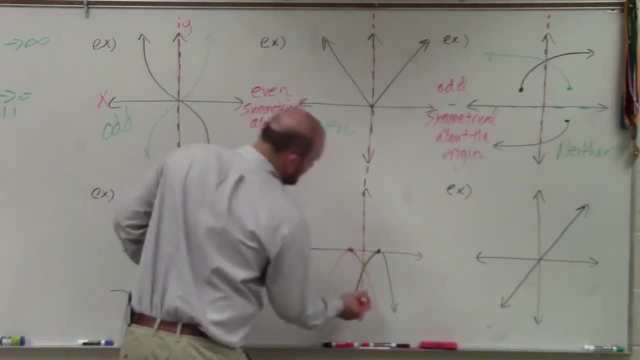 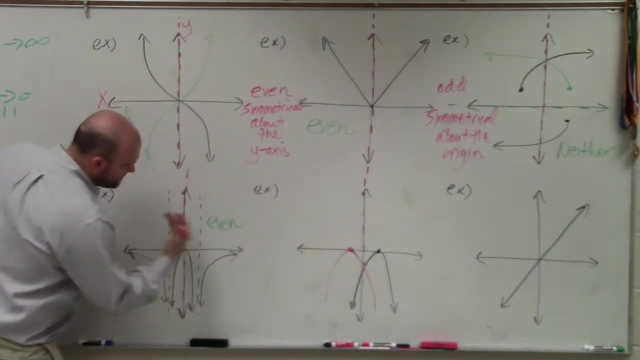 if I was going to reflect this graph, it's not going to produce the same graph. If I reflect it over the y-axis, it's not going to produce the same graph. When you reflect, you've got to have the mirror image of the graph.